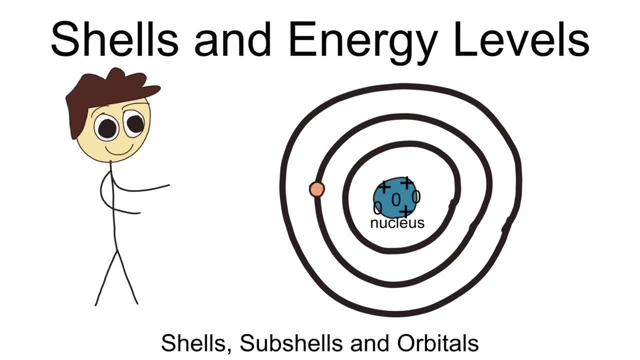 energy, because it takes more effort and more energy to pull electrons away from the center. We have labeled each of these circular lines, aka energy levels, simply as 1,, 2,, 3, and etc- Just FYI, the technical term for the numbers in 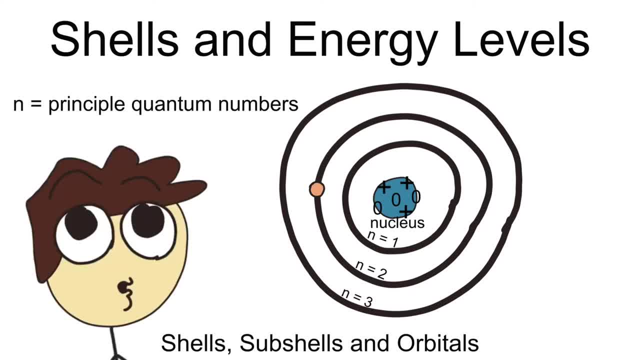 these energy levels is called the principal quantum numbers. We use the letter n to represent the different levels. The higher the n level, the further away it is from the nucleus, and the smaller the n level, the closer the energy level is to the nucleus. Also, the energy level closest. 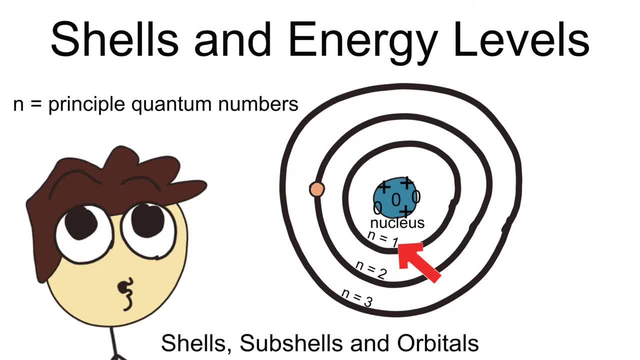 to the nucleus is valued at n equals 1.. Remember we're talking about Bohr's model, a simplified representation of the atom and all its parts. As you can see, the principal quantum number n is equal to 1,, then 2,, then 3, and so on. as the 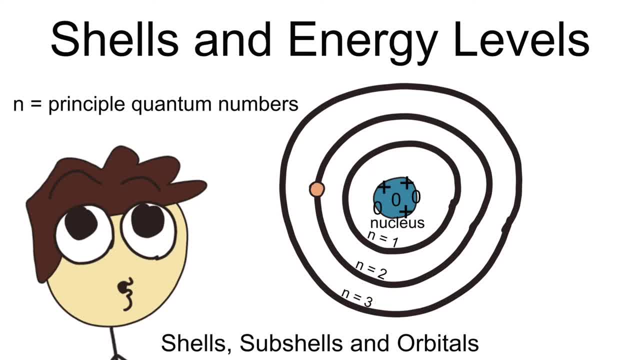 amount of energy is injected to push the elements further and further out. The electrons occupy lines circling around the nucleus. Sometimes you'll see that k, l, m and n are used instead of 1,, 2,, 3, and 4.. 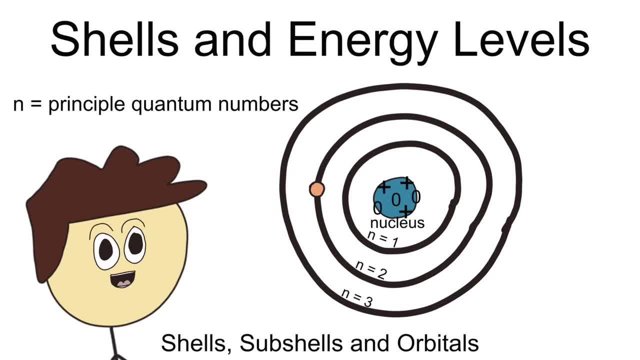 numbers, Because it's just easier that way And, as you can see, the further away you move from the nucleus, the energy increases. Now each energy level again- aka shells- can only hold a specific number of electrons total. for that example, The first energy level can hold up to 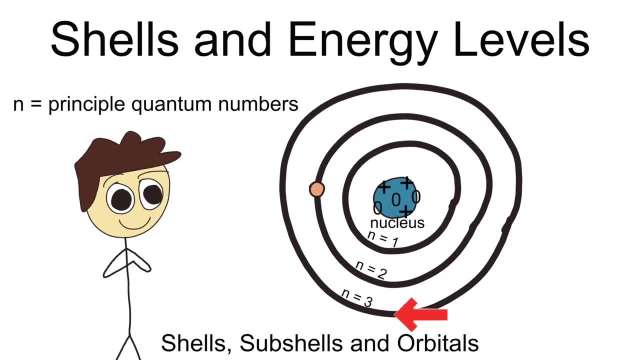 two electrons. The second can hold up to eight, The third is up to 18, and so on. There's actually a really simple formula to determine how many electrons an energy level can hold, but we'll talk about that later on. Okay, this is the nucleus right here in the center and the electrons 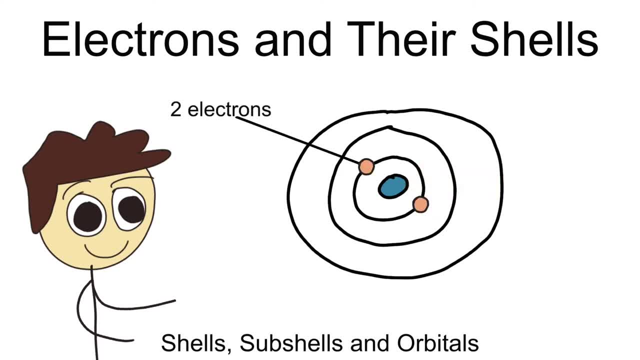 surrounding it. Notice that I mentioned earlier that the first shell, or energy level, has two electrons, the second has eight and the third and last shell on this picture has a total of 18 electrons that can occupy that space. It's a pretty good representation here, since the further out. 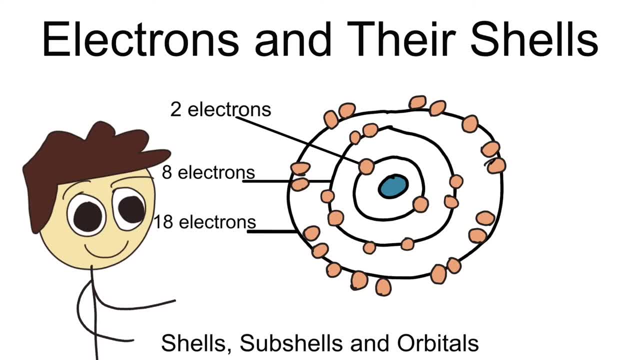 the circles are, the more space we have to hold. So let's take a look at the first shell and add electrons. You might be asking- or at least I hope you're a bit curious about this- what about the fourth shell? How many electrons can that carry? Going back to what I mentioned earlier, 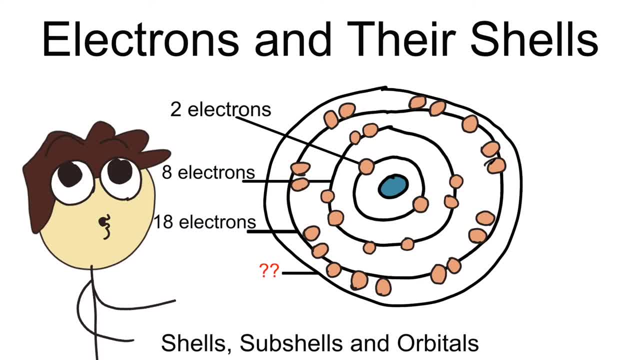 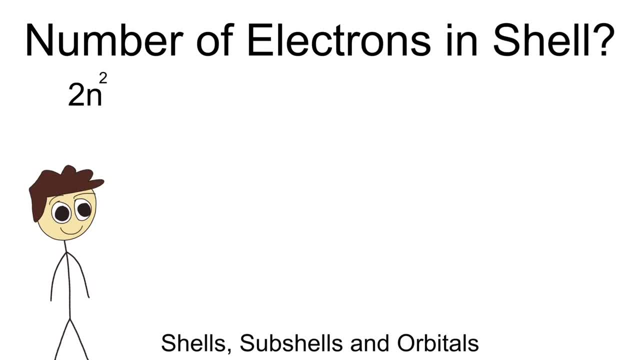 there's a very, very simple formula that allows us to predict the number of electrons that can fit into a shell. The formula is simply 2n squared. See: 2n squared would equal the maximum number of electrons that can fit in the shell. Using this formula, we can tell how many electrons will. 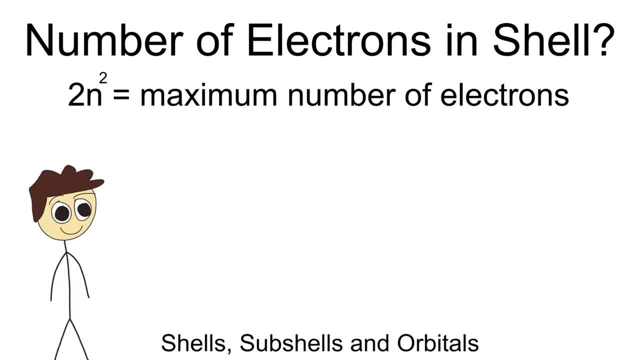 inhabit everything. So let's take a look at the fourth shell. Let's take a closer look at this formula. The n there refers to the shell or energy level number. Basically, if we were to ask how many electrons are in the first shell, n would be 1.. How many? 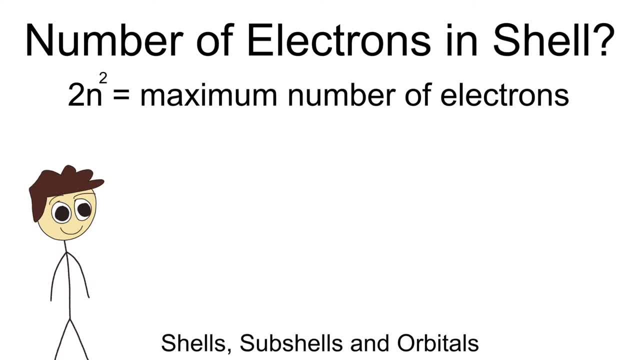 electrons are in the second shell, n would be 2, and so on. Simple enough. We already know from this video so far how many electrons inhabit energy levels 1 through 3.. Let's find out how many electrons can fit into the fourth shell, Since n is the number of electrons that can fit into the 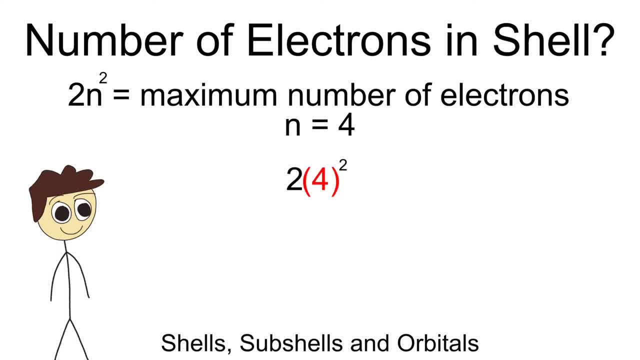 first shell, n equals 4, let's replace n with 4.. And according to the order of operations rule in mathematics there are two operations going on here. One is to square and one is to multiply. Since the order of operations rule applies, it tells us to square first, then multiply. So 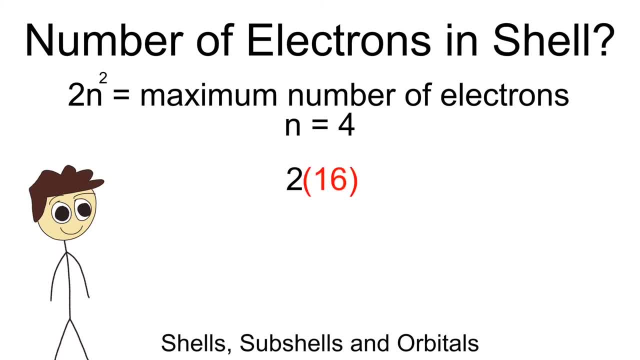 the shell, number 4, is squared, which is then equal to 16.. And then we simply multiply 16 to 2, and the answer is 32 electrons. That is the maximum number of electrons that can be held in the first shell. So let's take a closer look at this formula. Let's take a closer look at this. 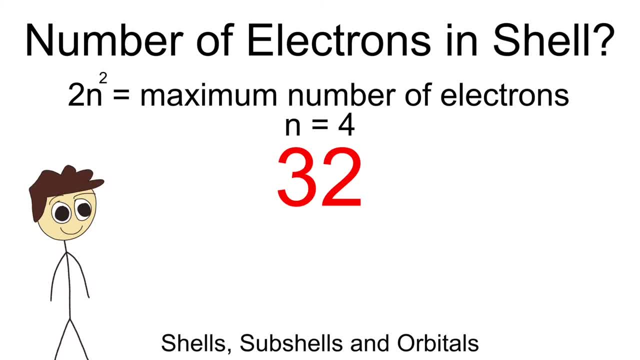 in the fourth shell. Let's confirm this by figuring out the maximum electrons the second shell can carry. Again, the second shell would make that n equals 2.. Now if we calculated 2 squared, then we get 4.. And 4 multiplied by 2 is 8.. Fantastic, It works. Okay, let's move on to. 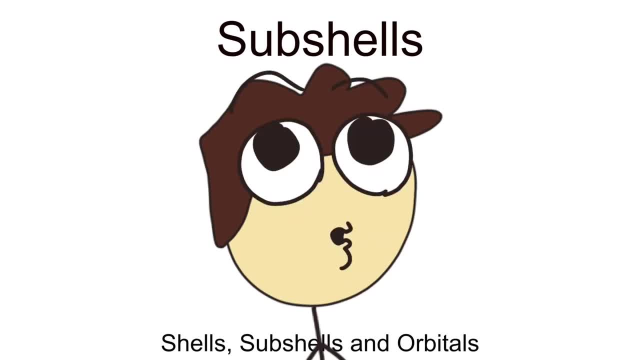 subshells. Try and guess the relationship between shells and subshells. If you guess that subshells are pretty much smaller shells within normal shells, you're kind of halfway there And, like always, we need to label these things. So what do scientists do? They give subshells. 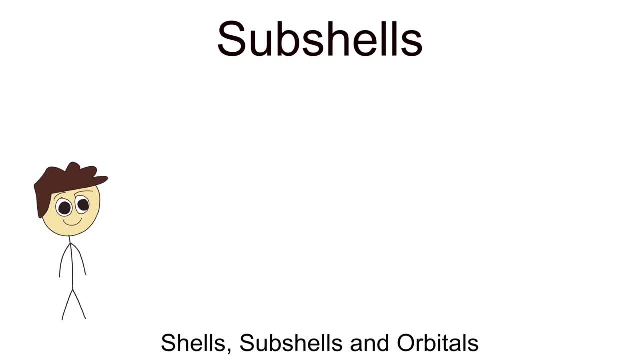 letters to reference itself as a subshell. You're going to have to remember this, but I'll try to explain it in a way that's simple to understand. So, within each energy level or shell, there are sublevels or subshells, And, fortunately for us, there are only four types. 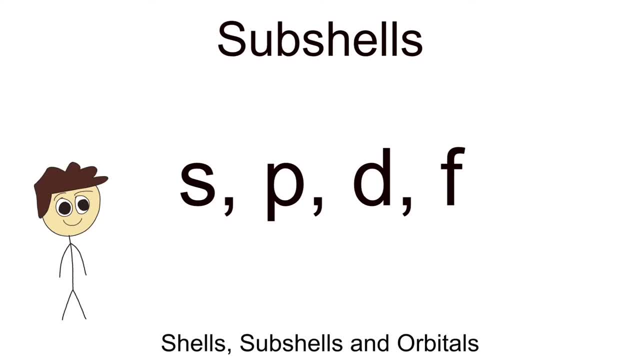 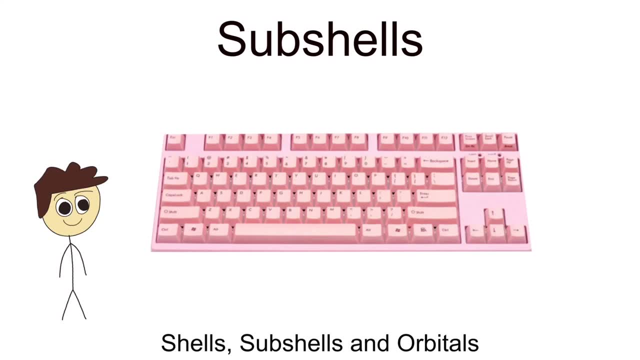 S, P, D and F. This is a silly way to remember it, but I'll just show you guys how I remember it. Look at your keyboard on your computer. Just take notice where those letters are and how you would type: S, P, D, F. That's basically it. Whenever I try to remember these letters, I just remember. 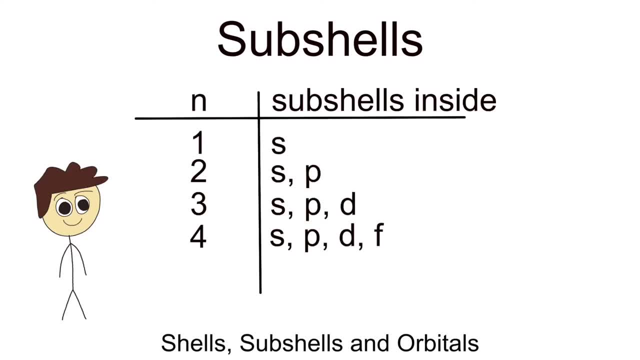 the keystrokes I make. It's kind of weird, but that's how I learned it. So if you look at the table, I like to think of it as an award system. On level 1, or n equals 1,, you are given an S. 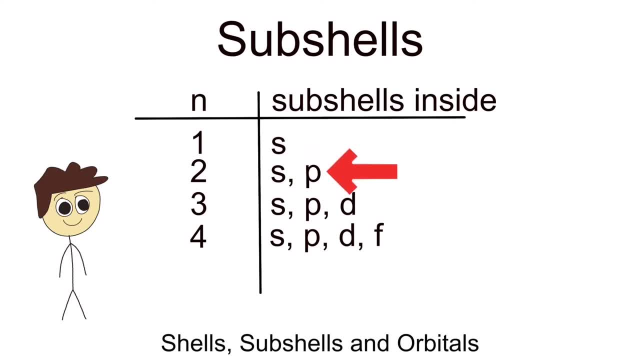 Once you move to level 2, you already have an S and are given the letter P. If you continue on to level 3, you got the S, P and D. Now one pro tip is just to notice how the n number actually. 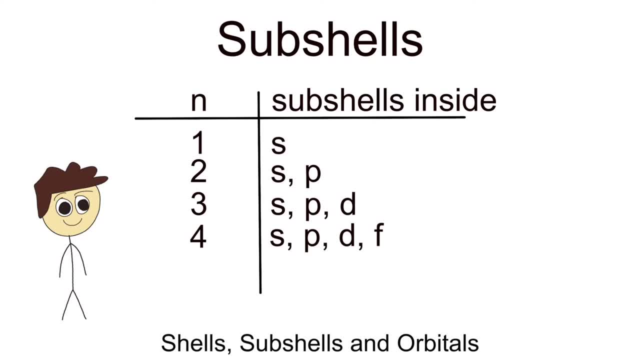 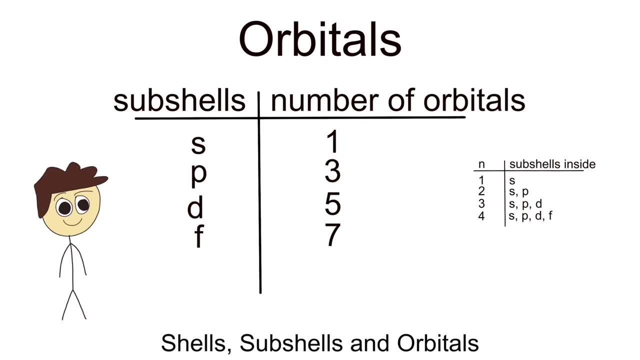 equals how many sublevels you have. It's a neat little trick to keep in mind when you're trying to remember this. Now, within each lettered sublevel, there's something we call orbitals. Orbitals are pretty much precisely where you find the electrons. 90% of the time, Each orbit can 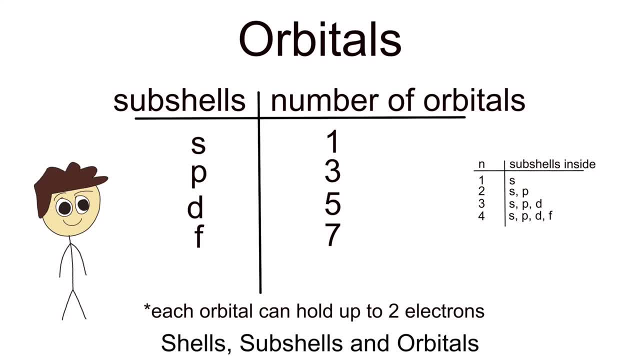 hold up to two electrons. Remember that two electrons. Sublevel S has two electrons, So one orbital. Sublevel P has three orbitals. Sublevel D has five orbitals And F has seven orbitals. It's just odd numbers there, from 1,, 3,, 5, and 7.. Since each orbital can hold up to 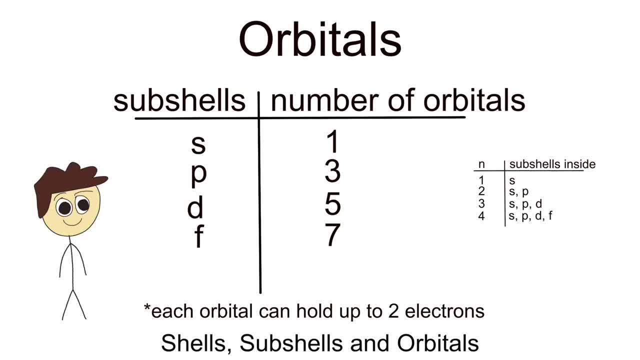 two electrons. that would mean that sublevel S, with its one orbital, has two electrons, while P has three times two, which is six electrons. D has five times two, which is 10.. And F has seven times two, which is 14 electrons that it can hold in that single. 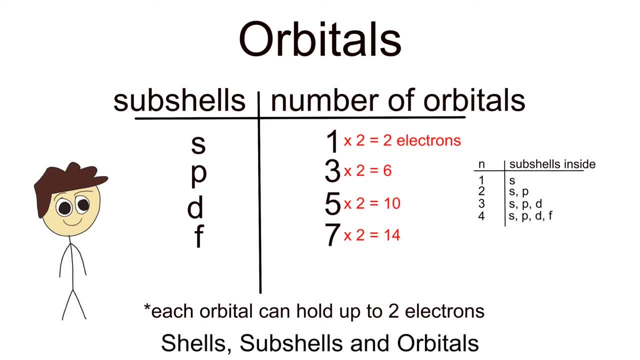 sublevel. Keep in mind that these are subshells, not shells themselves. Depending on the level of the shells, it can contain more than one subshell, like how shell number four has subshells S, P, D and F. I tried to think of a way to explain this in a broad perspective and I think the